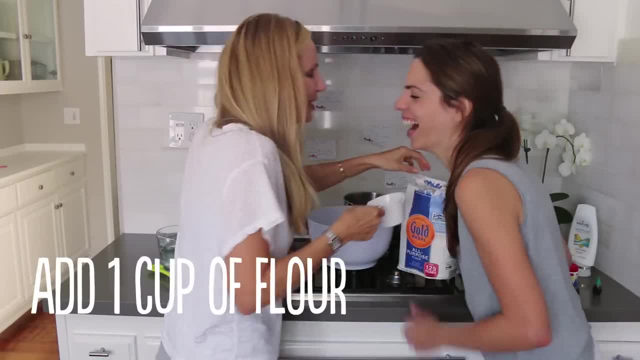 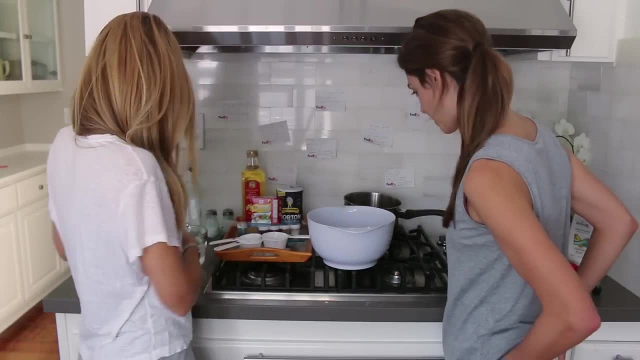 How do we get the flour in here, though? Do you just like scoop it out, Meg, Come help us. That's about it. About a cup, About a cup. About a cup Okay. About a cup of flour, Okay. 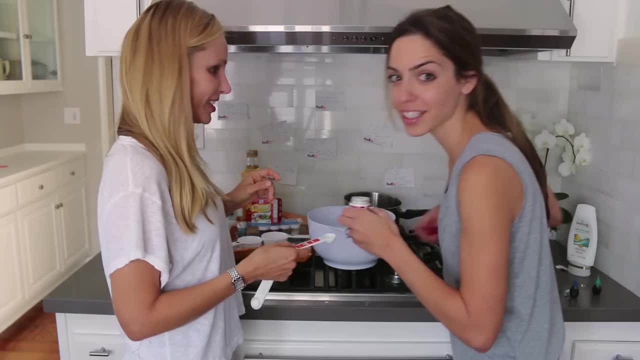 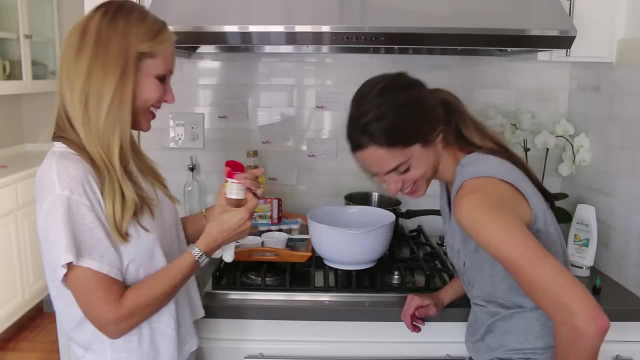 And a fourth cup of salt, And then cream of tartar. Oh, Interestingly enough, cream of tartar is a powder. I know. I spent a lot of time in the non-powdered food aisle looking for the cream of tartar. 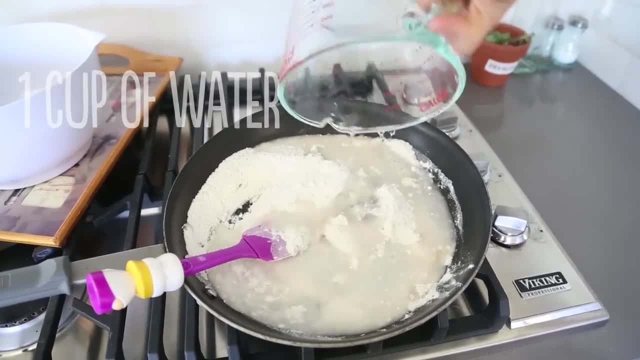 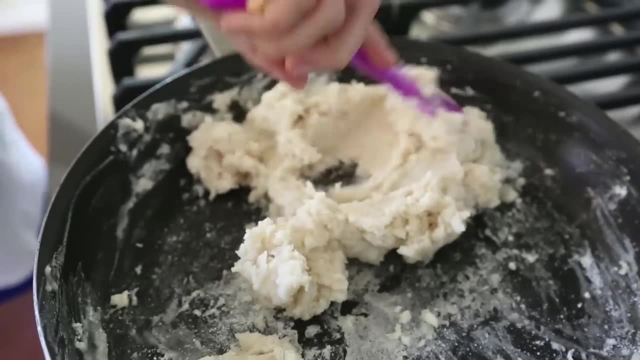 Should I back up with Brooke in the kitchen? I'm a little nervous. You probably should be. It looks great. I mean, it's looking like Play-Doh. This looks like Play-Doh. It's hot, you Yes. 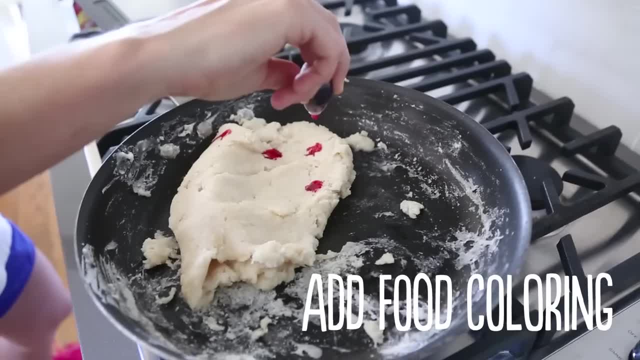 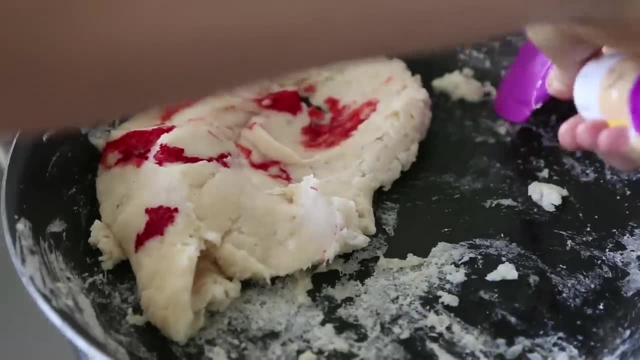 Woohoo, Let's put the food coloring in now too. Why not? Why not? It looks like the Play-Doh is bleeding. Oh Help me, Help me. That does not look appetizing. What Are we just dumping it like this? 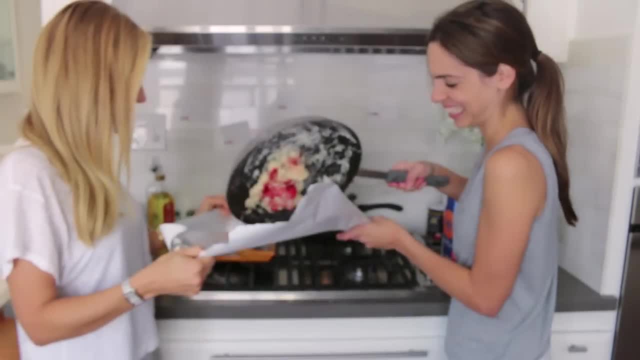 Oh Okay, so now we are kneading this warm dough. It is actually rather enjoyable. It turned out pretty nice. No glitter, No matter how cute it looks on Pinterest, Just no Resist the urge. It worked. It worked. 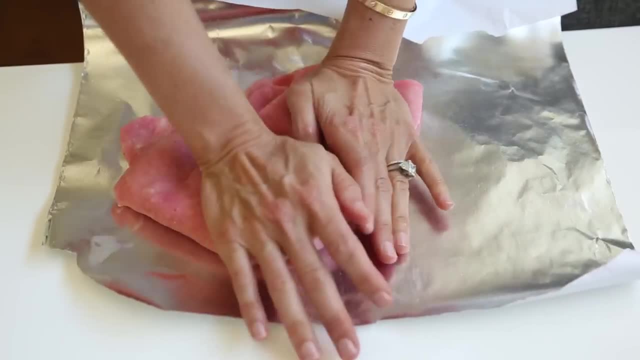 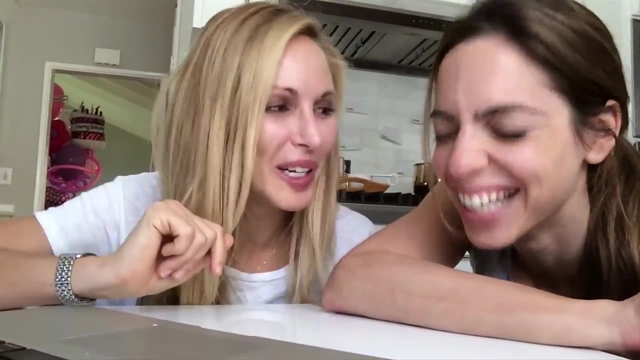 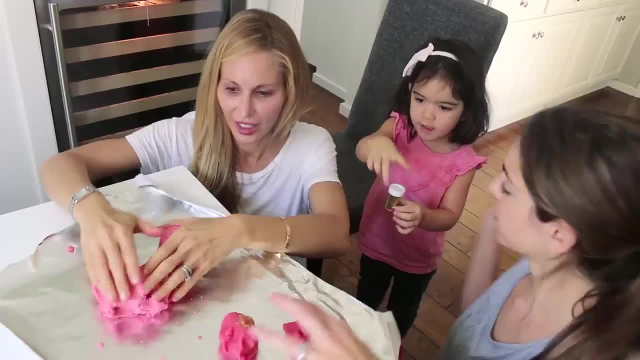 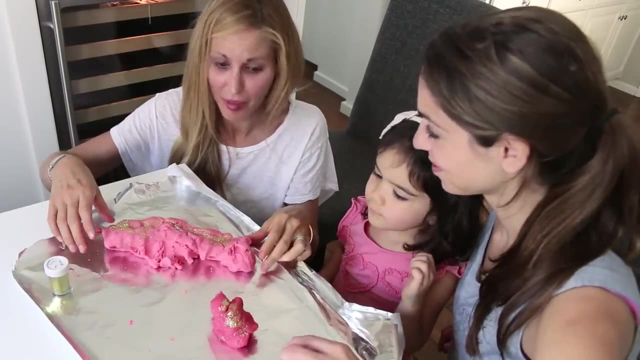 Oh my gosh, Oh gosh. It's so pretty, though So beautiful. The gold, What's that? It's glitter. Oh, This is really cool, Jennifer, I don't know. My life is really good right now. 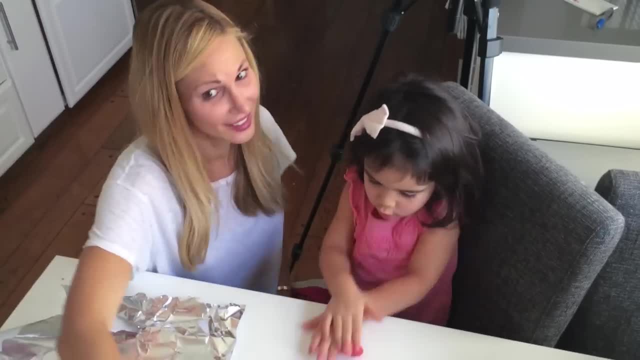 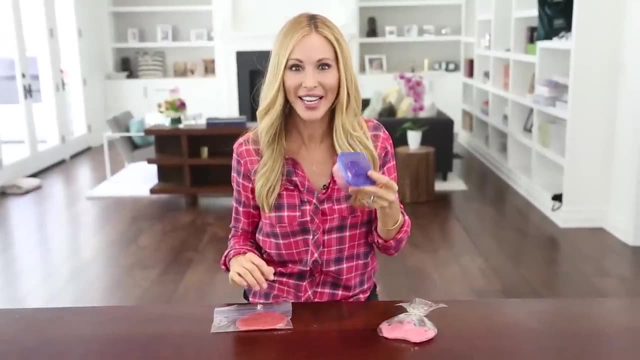 I mean, I may be agreeing with you in a couple hours, but right now life is good. Success Mm-hmm. I hope you guys will give this a try. You can either store it in a Ziploc bag, or I really like these small airtight containers. 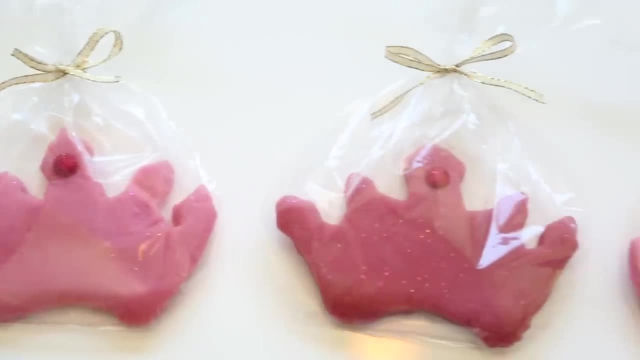 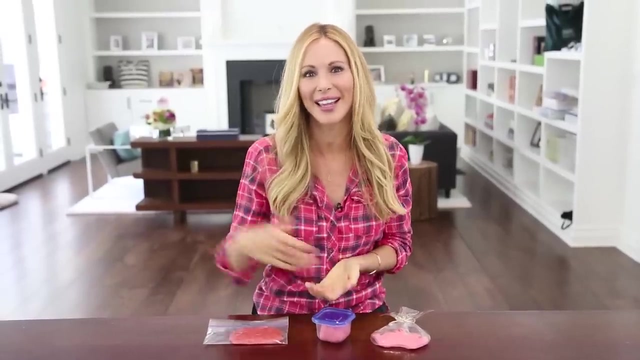 But since we are doing these for Presley's birthday party favors, we cut them into the shape of a crown with a crown cookie cutter, and I think they turned out so cute. So thanks for watching, Don't forget to subscribe and I will see you next Friday. 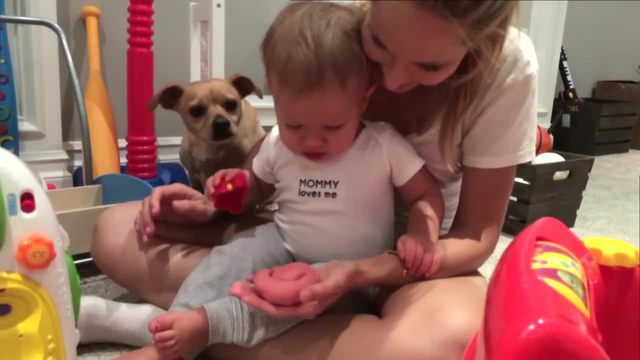 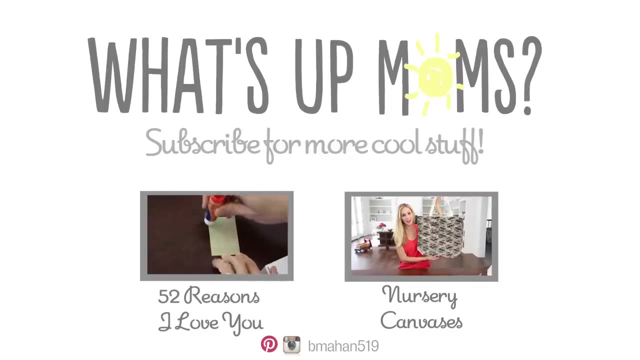